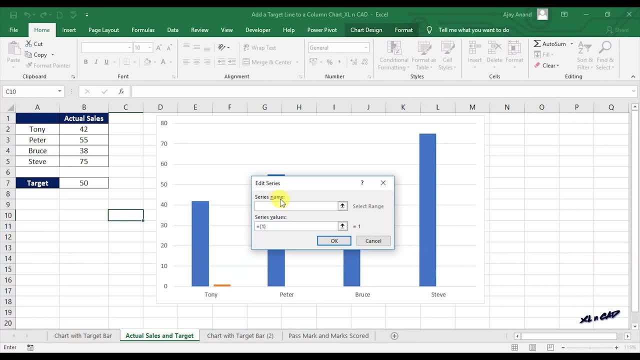 in the series name, or else you can specify the cell containing the text for the series name, Then select a série data in the target line. In this case, I will select this cell A7, which contains the text target. Now the Series values. Let me delete the existing data and I will select the cell B7, which 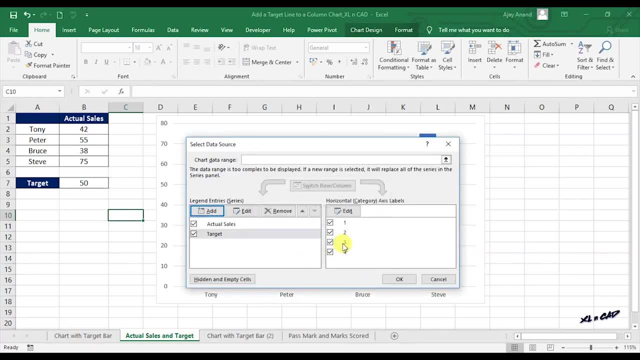 contains the target figure. Click okay Once again. click okay, Ok. Now we have a column representing the target figure. To change this chart type, click the воспly column of the target field and select the column representing local target field. 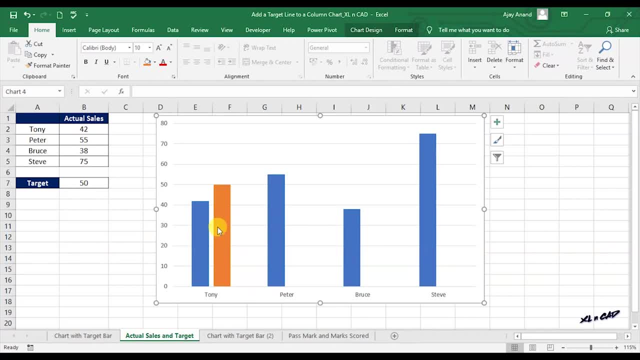 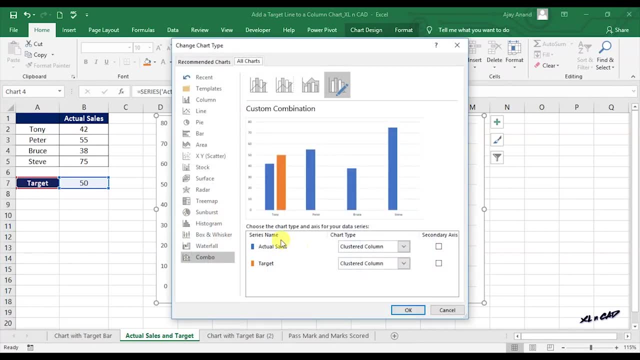 Click su. Click adopt, Click ok, Click ok. Now we have a column representing the target figure. To change this chart type, choose the right-click on the column, select change series chart type. now we have the dialog box for available chart types, both the data series and the type of. 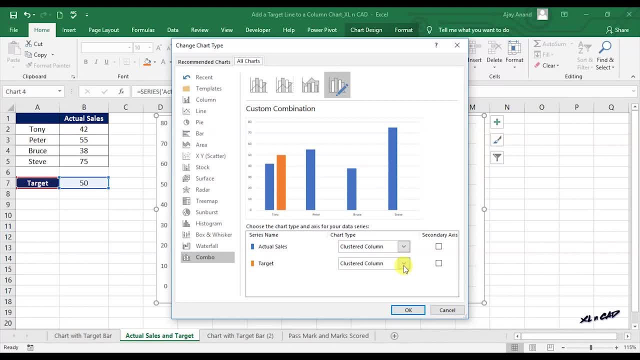 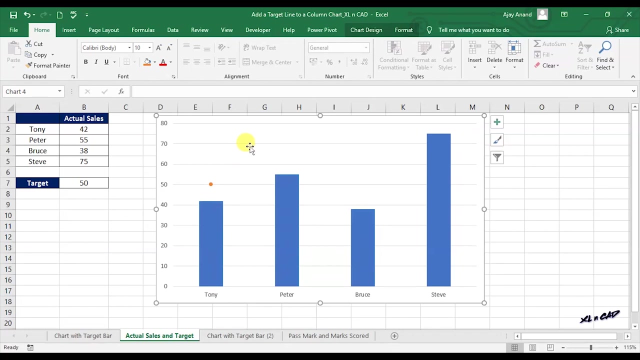 charts used are listed here. click on the drop-down menu against data series: target. select scatter chart. under XY scatter, the column that represented the target figure has now become a point. now we have to add error bar to this point. before that, I will delete these grid lines for adding an error bar to this point. 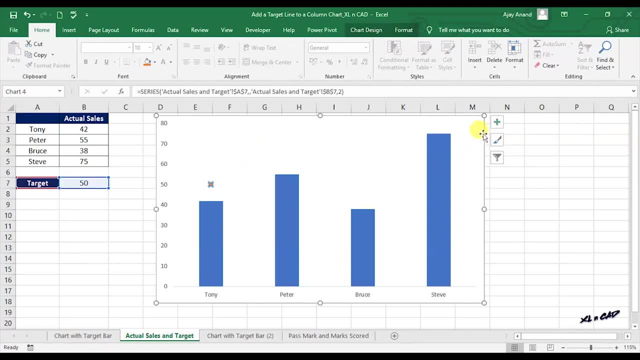 select the point. click on the green plus button for chart elements. mark the checkbox for error bars. to format the error bar, right-click on the point. select format data series. in the task pane for format data series, click on this small down arrow against series options. select series target X error bars. 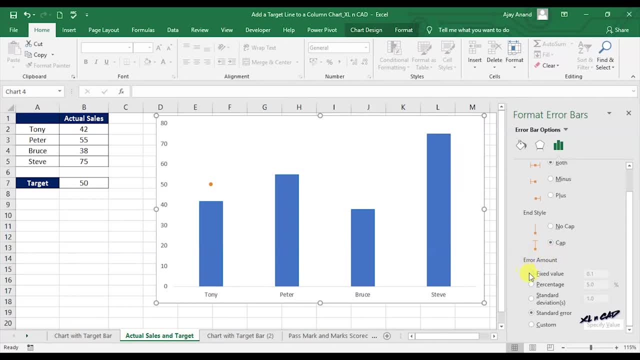 here we have to specify the error amount and this value determines the length of the target line. of the target line, we can assign a value to the target line. we have four entries here and I will use the value 4, and this is the error bar which will represent the target line right now. the 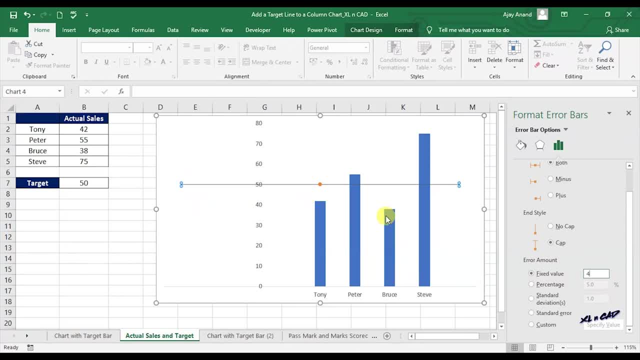 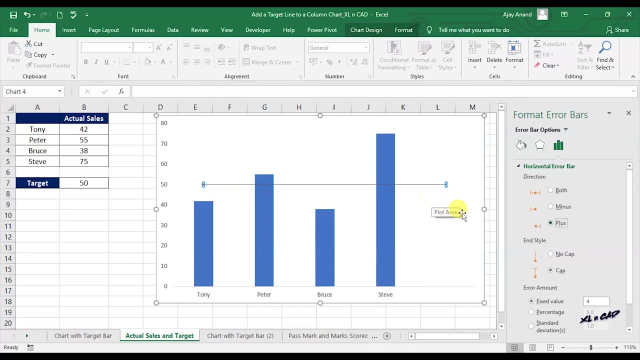 line is not within the required limits, so let's apply some formatting. select the radio button against plus, then no cap. click on the fill and line option for changing the color and line type. I will change the color of the line to red. will increase the width of the line. 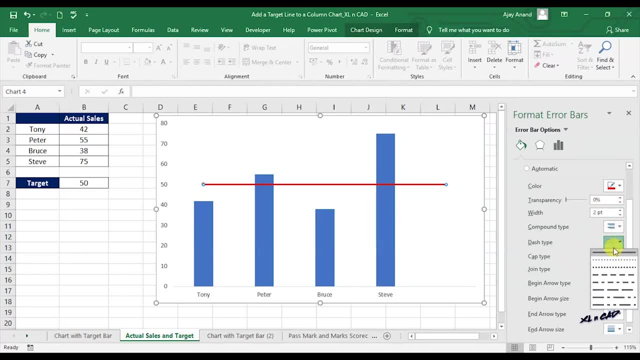 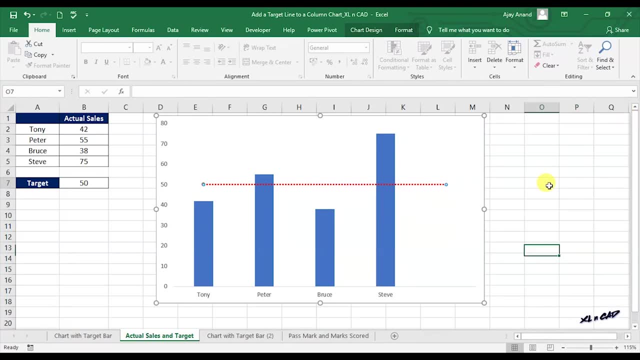 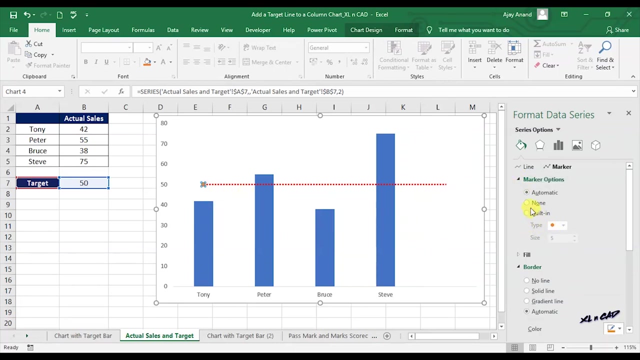 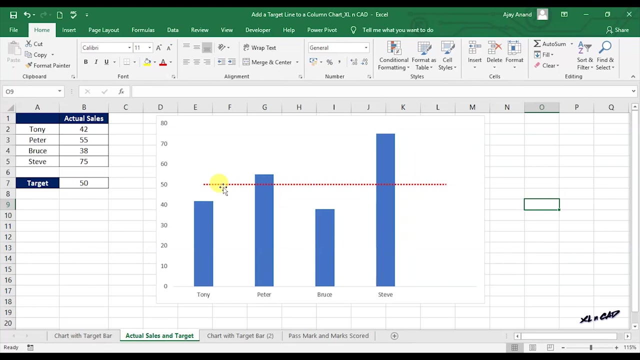 We can also change the line type here To hide this marker representing the point. right click on the point. format data series: fill and line marker under marker options: Select none. Now the marker is gone. Now we have to position this line for that. right click on the line. select data select. 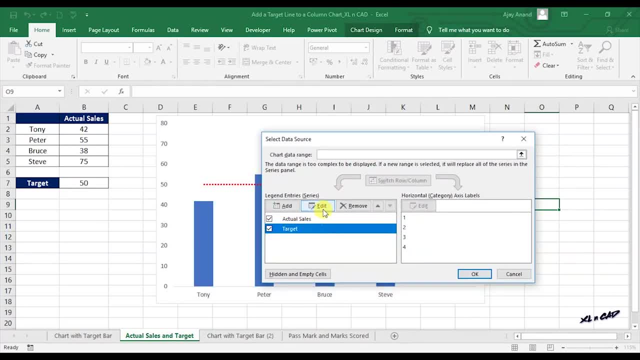 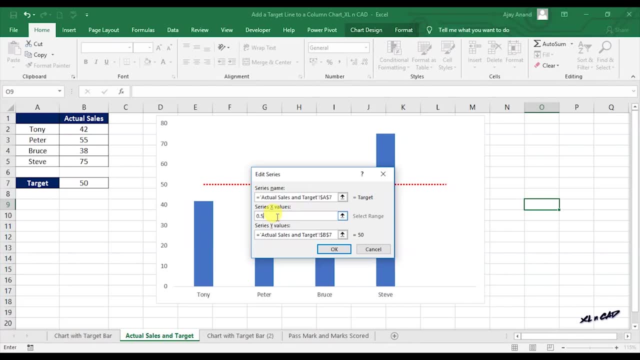 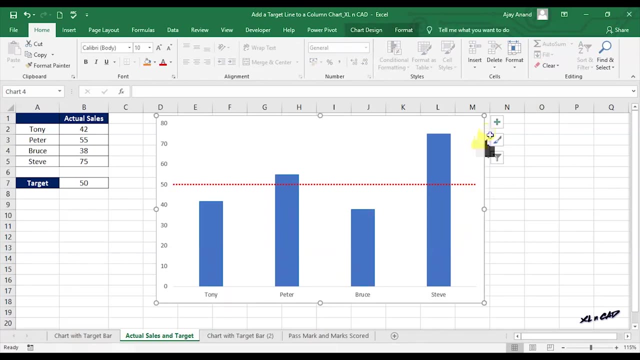 the data series target edit type in 0.5 in the input box for series x values And this will reposition the target line. Click ok To add data label. mark the checkbox for data labels. Let me move this label here. 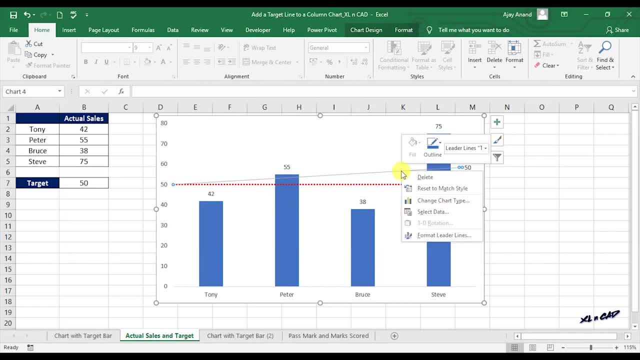 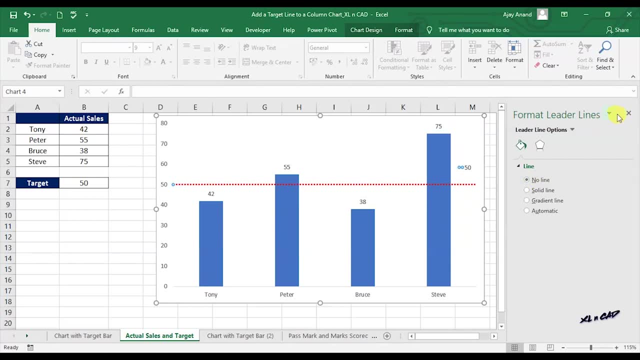 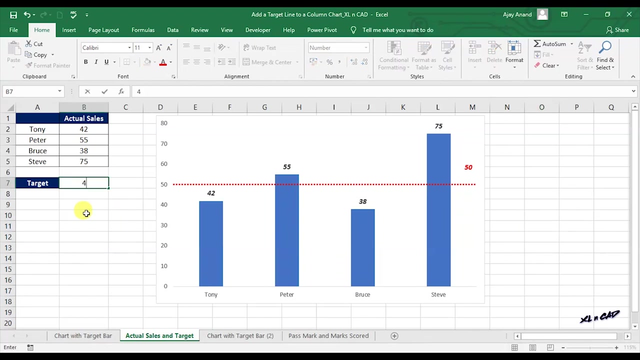 To hide this leader line. right click on the leader line format leader lines. select no line. I will quickly apply some formatting to the data labels And this is our column chart with a target line And when I change the value here in this cell, the position of the target line will update. 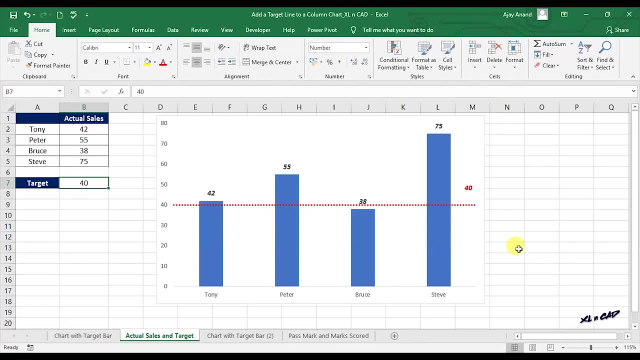 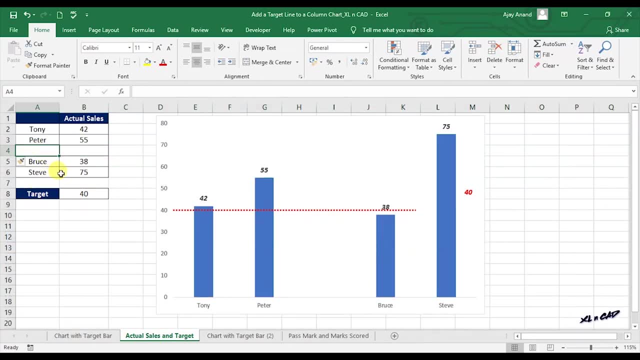 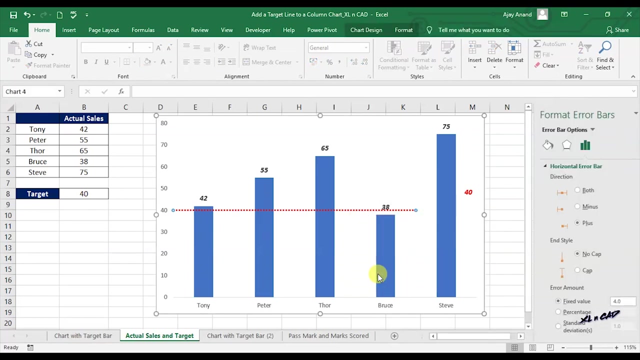 for that change. If you want to make a new entry here, Insert a new entry, Insert a new row and type in the data, And here we have the column representing the new entry. Now to increase the length of the target line, right click on the target line format error. 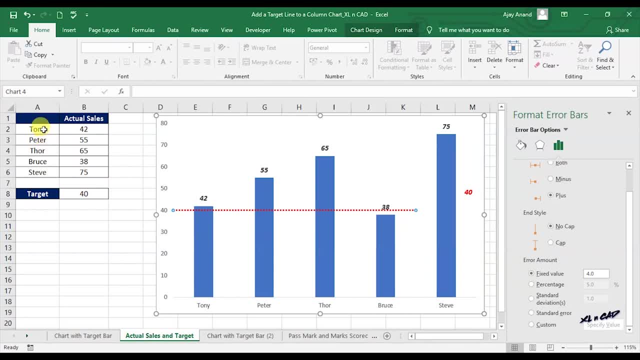 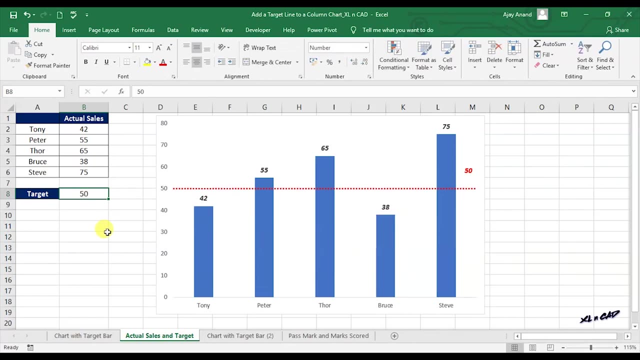 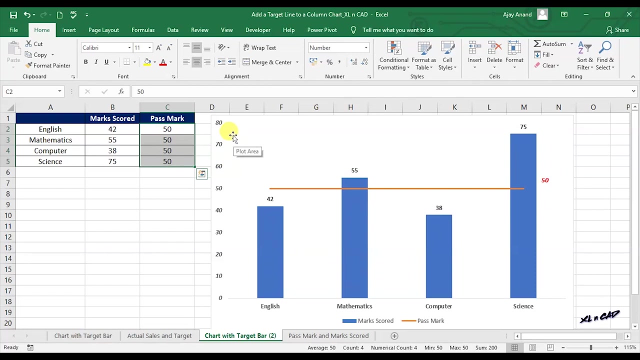 bars. use the value 5 instead of 4.. Now the target line looks perfect. Now one more quick method for adding a target line to a column chart. This chart here is somewhat similar to the previous one and quite easy to make. 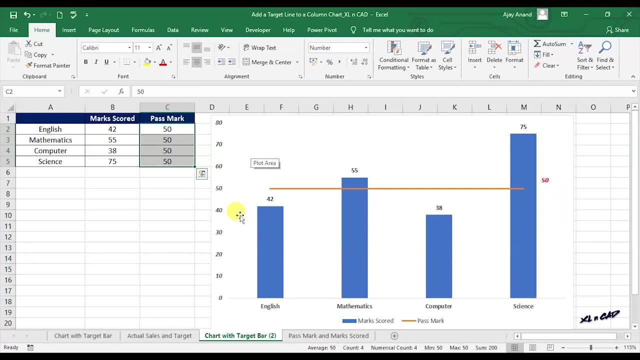 When I say easy, we can create this chart in less than a minute. But the disadvantage is we need to keep an additional column like this, which has the same value in every cell. That means if you want to raise or lower this target line. 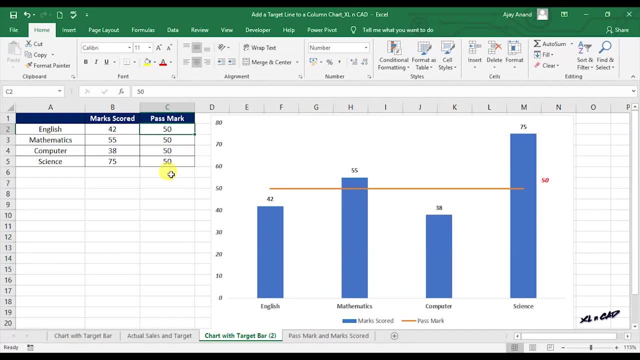 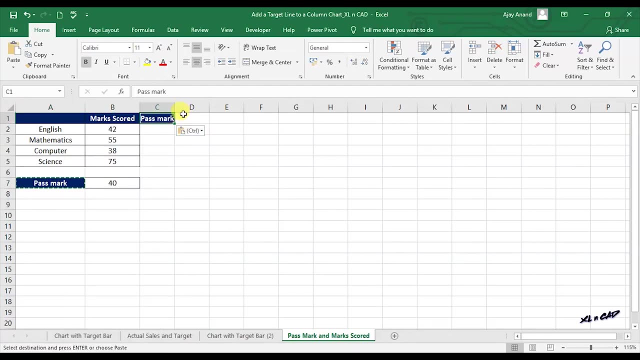 You need to change the value in every cell in the second data series. But I have a solution for this problem, So let me quickly show this second method. I will copy this cell here. will make an absolute reference to the cell B7, copy this formula. 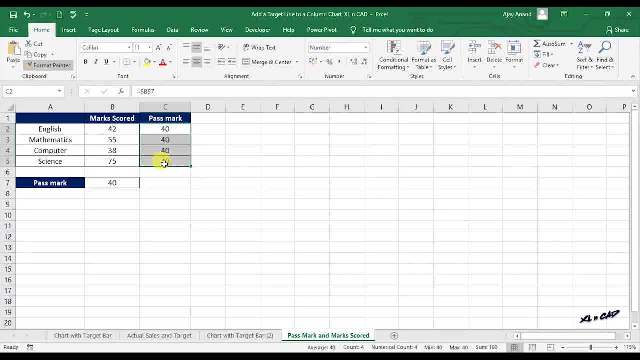 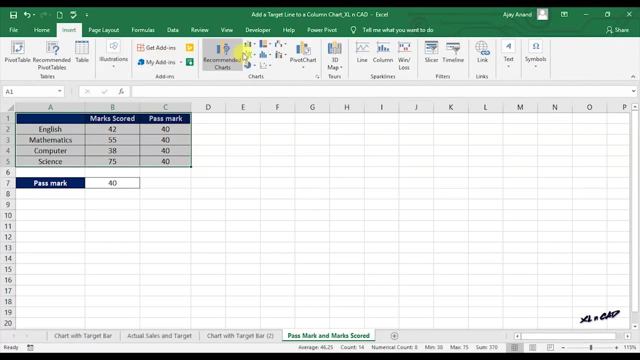 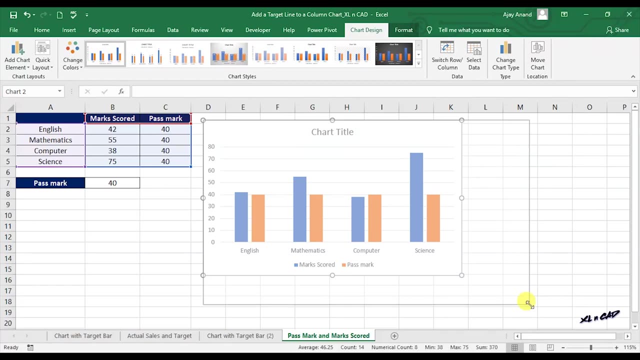 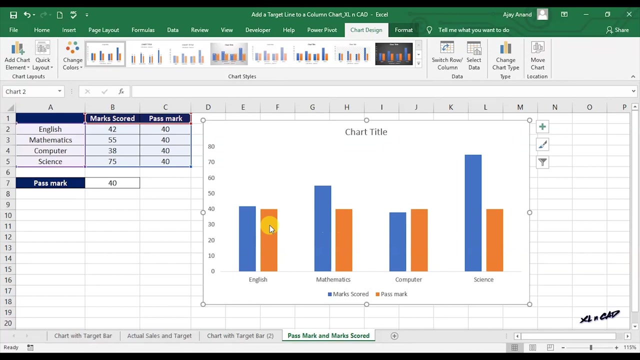 to the cells below For creating the chart. select the data. go to insert tab. insert a clustered column chart. The blue columns here represent the marks code and the orange ones represent the pass mark. Now I will change the chart type of the second data series, that is, pass mark. 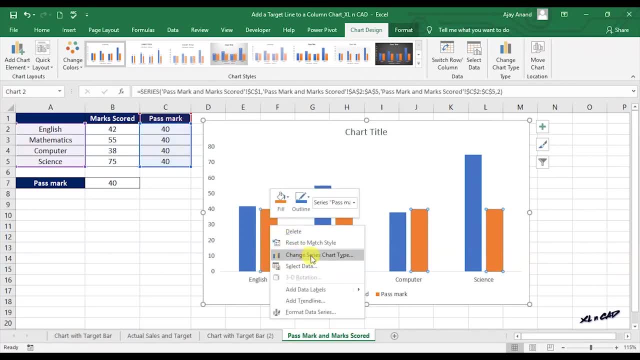 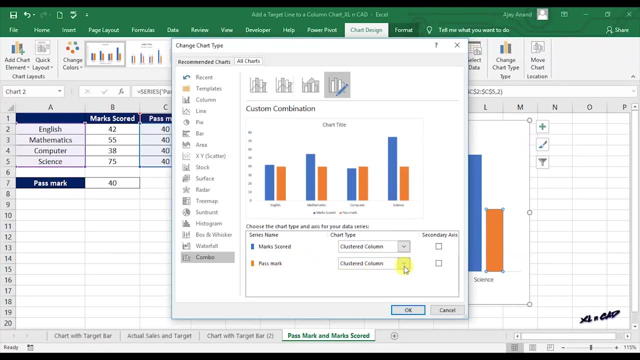 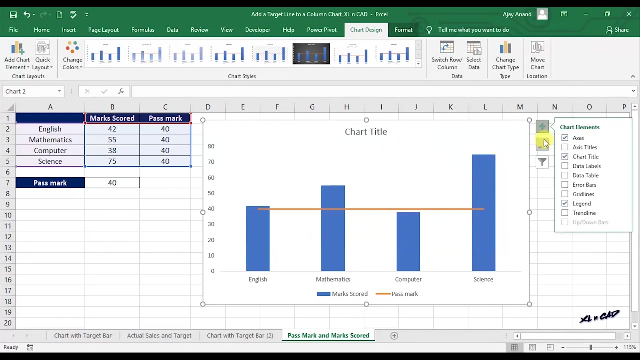 For that, right click on the column select. change series chart type. Click on this drop down menu against the data series. pass mark Select line. Again we have a column chart with a target line. Let me add the data labels.